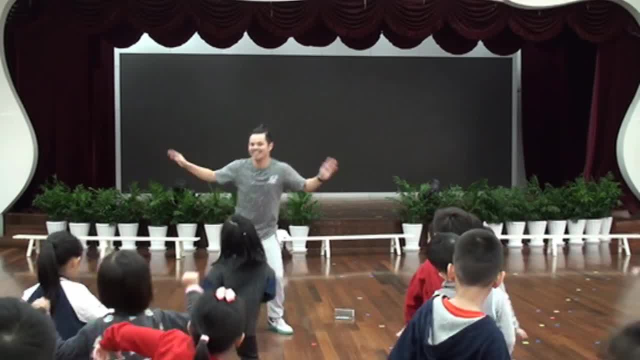 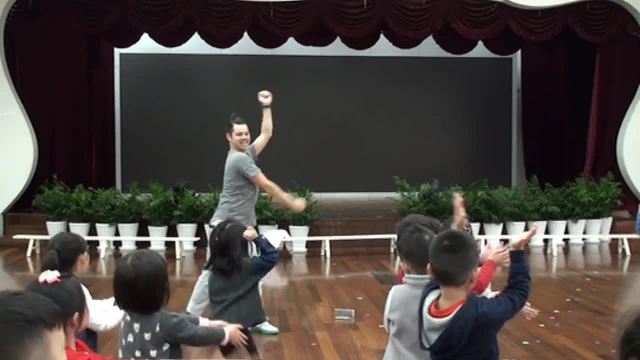 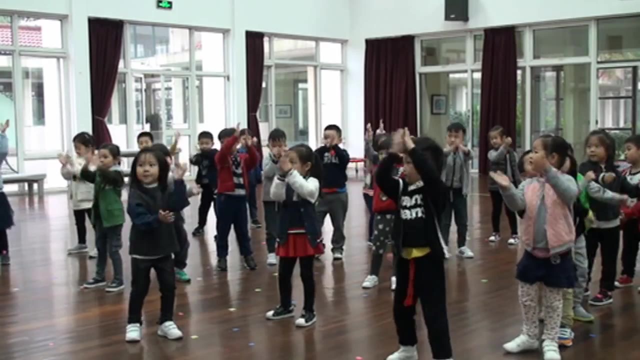 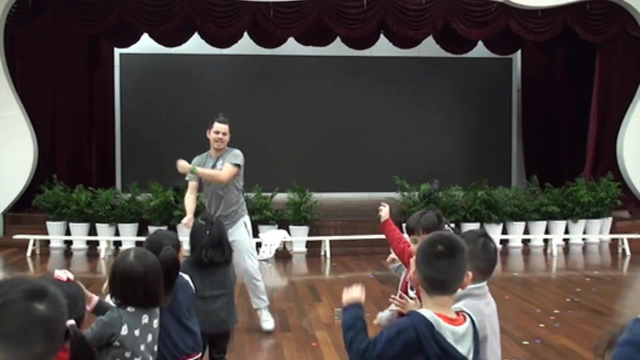 Nobody learns without getting it wrong. I won't give up. no, I won't give in Till I reach the end and then I'll start again. No, I won't leave. I wanna try everything. I wanna try even though I could fail. I won't give up. no, I won't give in. 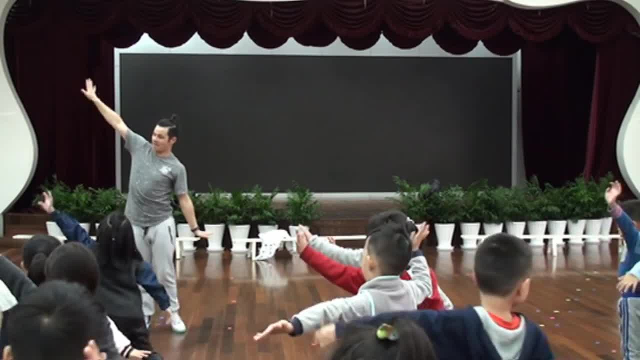 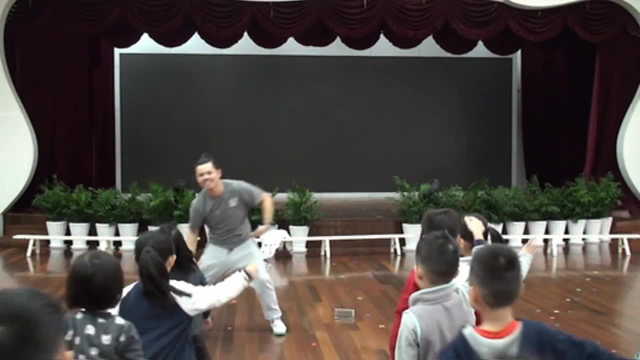 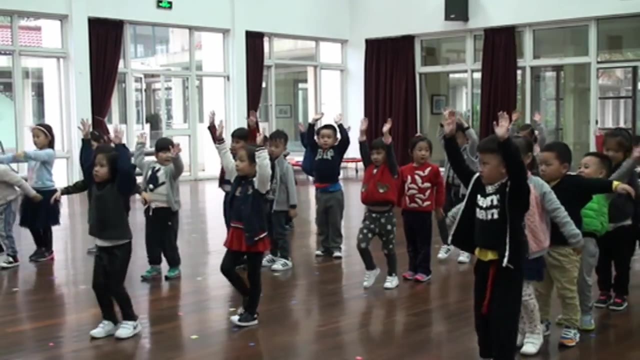 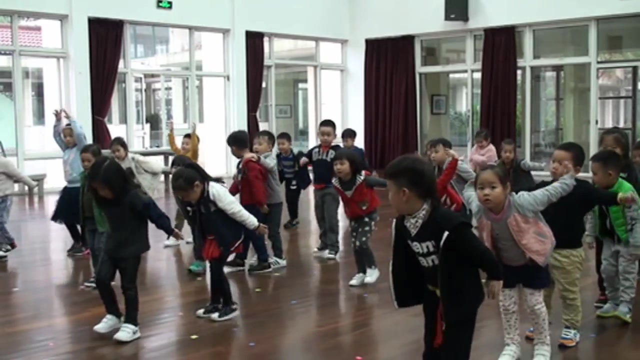 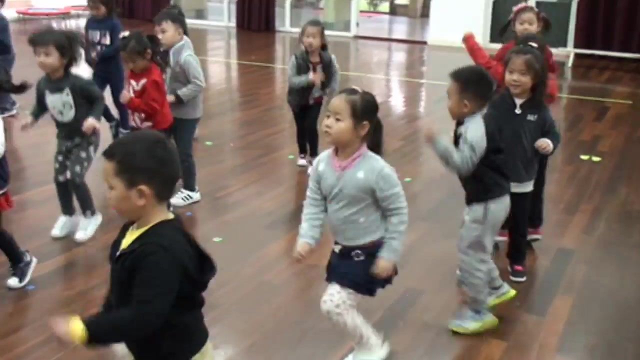 Till I reach the end, and then I'll start again. No, I won't leave. I wanna try everything. I wanna try even though I could fail. Try everything, Try everything, Try everything. Look how far you've come. You filled your heart with love. Maybe you've done enough. 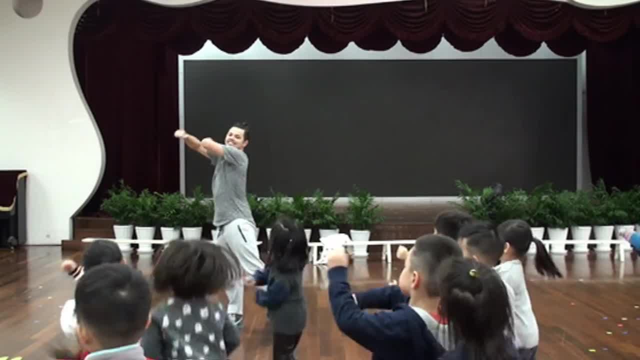 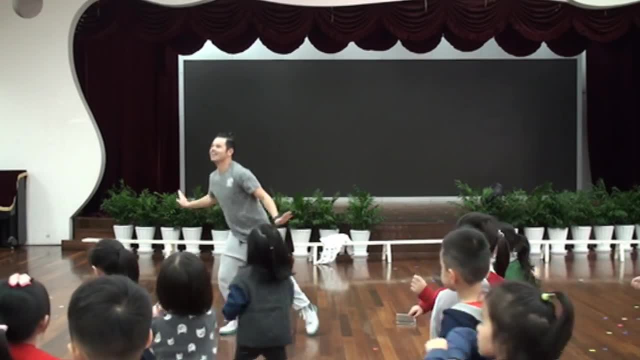 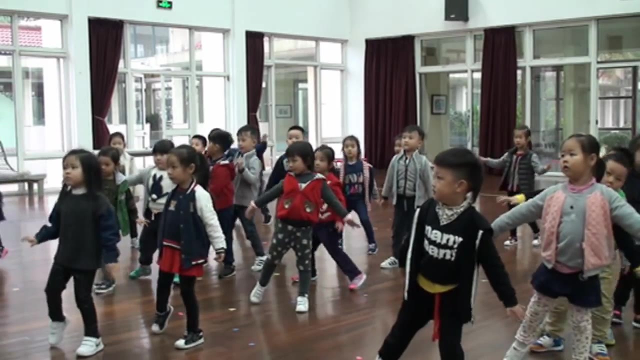 Take a deep breath. Take a deep breath. Don't beat yourself up. No need to run so fast. Sometimes we come last, But we did our best. I won't give up. no, I won't give in Till I reach the end, and then I'll start again. 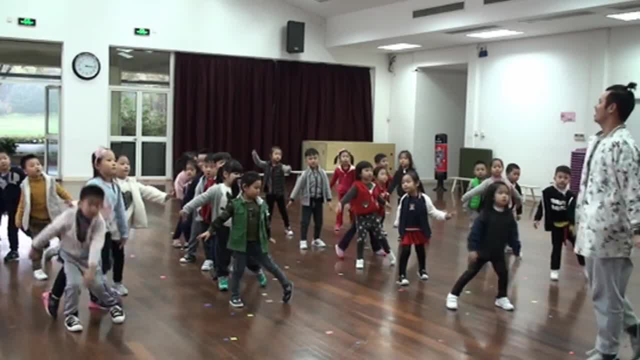 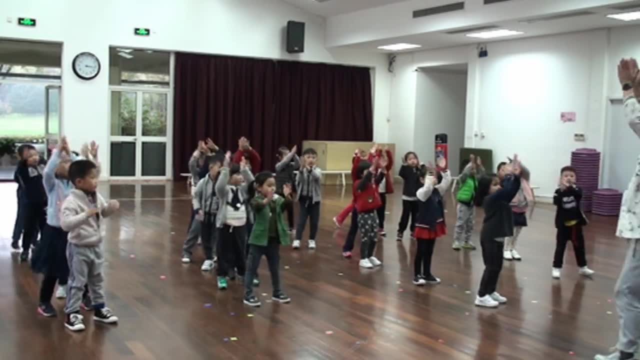 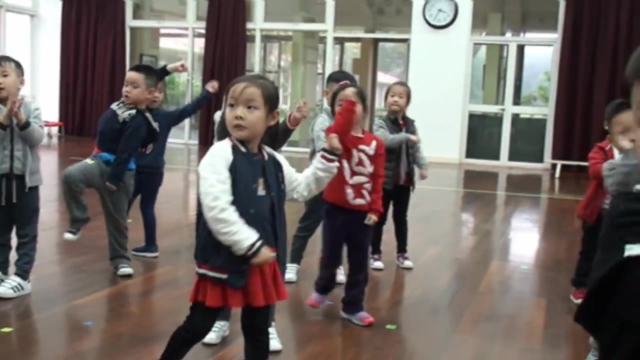 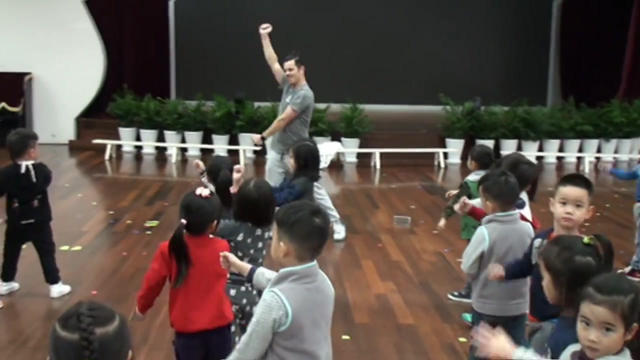 No, I won't leave. I wanna try everything I wanna try, even though I could fail. I won't give up. no, I won't give in Till I reach the end and then I'll start again. No, I won't leave. I wanna try everything I wanna try, even though I could fail. 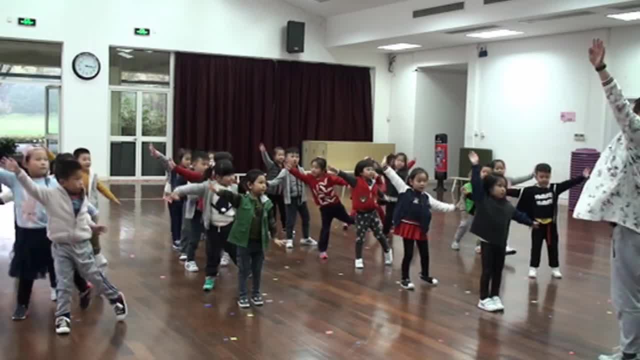 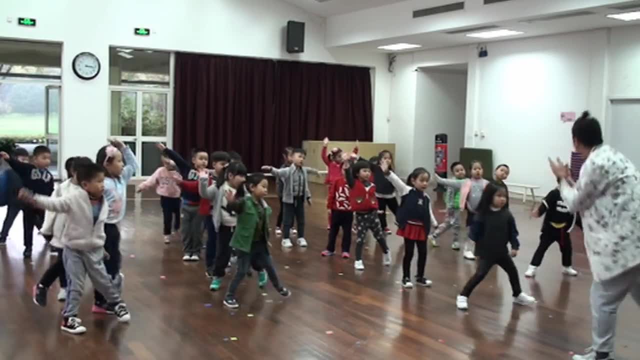 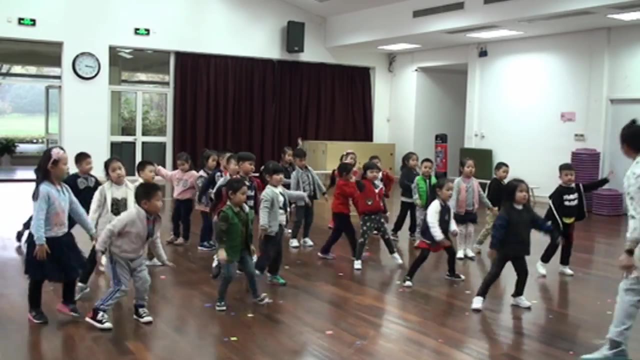 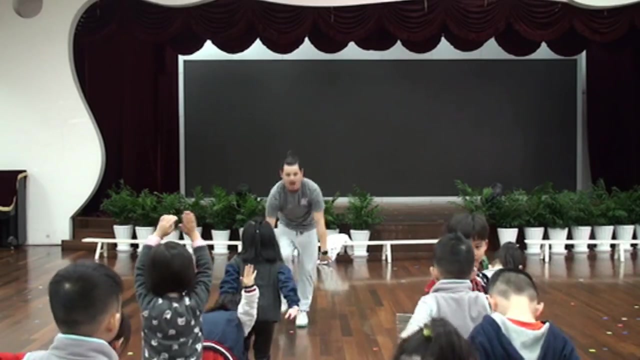 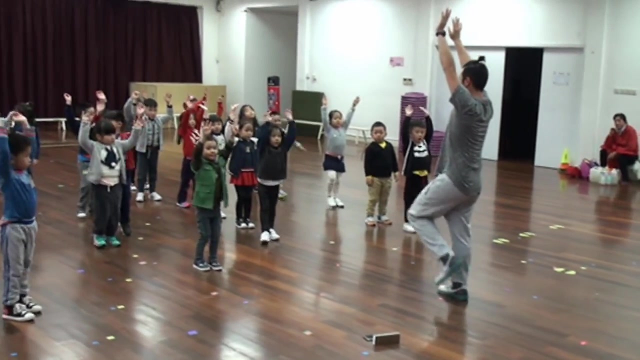 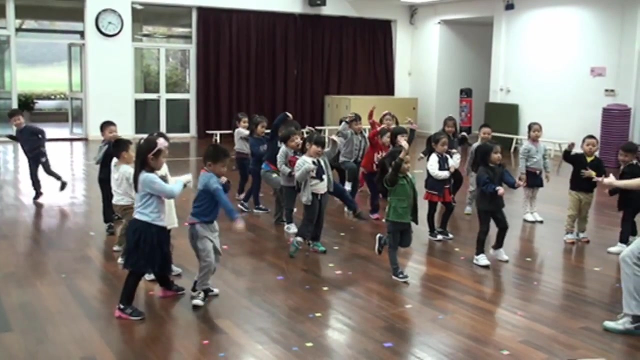 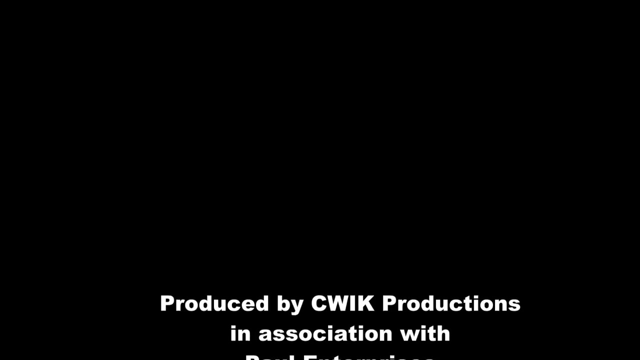